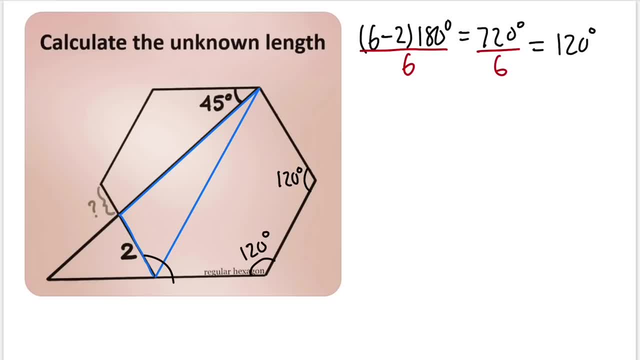 120 degrees. Likewise for this, this and the rest. All right, let's see, All the sides are the same. so we know this is congruent to that And because of that we actually know that this angle, it's the. 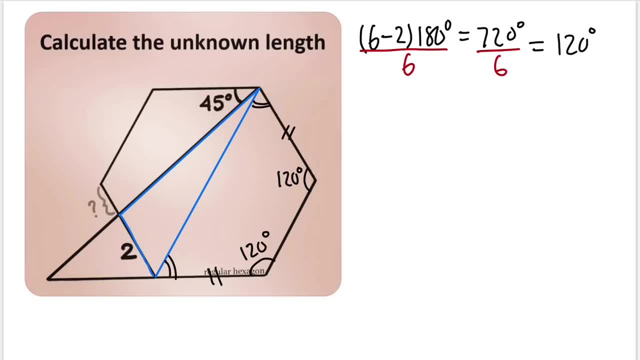 same as that angle. Well, how do we figure that out? then, Check this out. I know that this and that together is 120 degrees, and another 120 degrees already For this part. it's a trapezoid, technically, which the inside is 360 degrees, So just do 360 degrees. 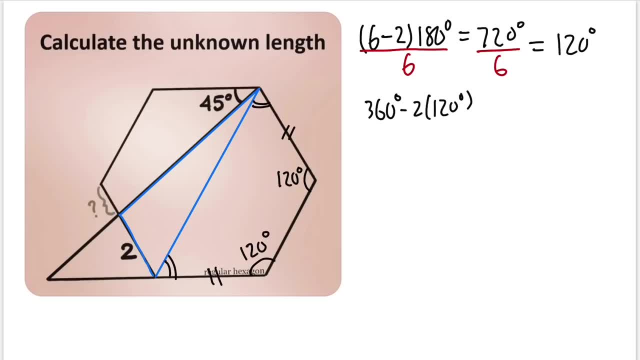 minus 2 of the 120 degrees and then divide by 2.. On the top is 360 minus 240, which is 120,. divided by 2, we get 60 degrees. So this angle is 60. likewise, this angle is also 60 degrees. 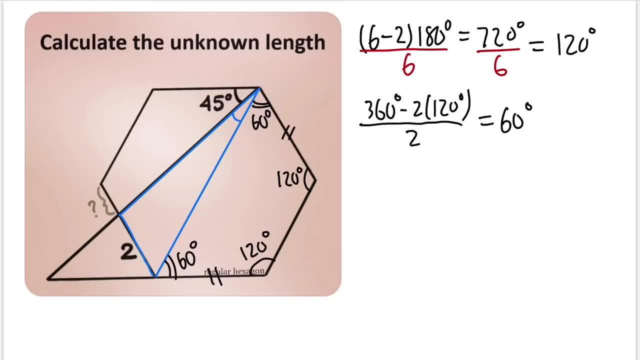 that said, we can actually figure out what this angle is to do. so we know the whole thing from here to here is 120. so let's just do 120 minus 45, minus 60, we will get 15. so that's 15 here. and then for this angle here, well, 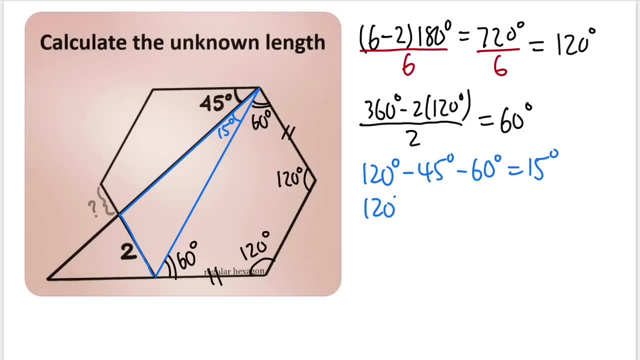 from here to here is 120, and then- we know this right here- is 60, so just minus 60 degrees, so we get 60 degrees and that's right here. and for this one right here, we know the blue triangle, the angle sum is 180. 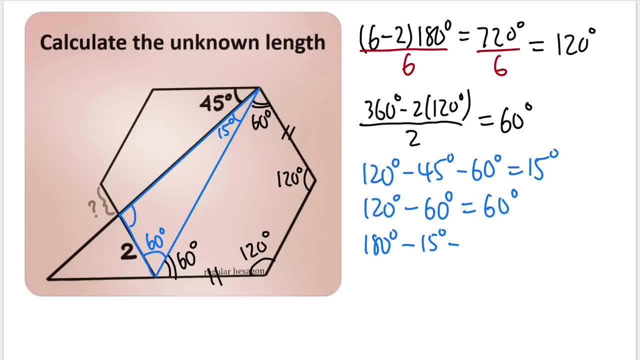 so just minus 15 and then minus 60, we will get 105. so just like that. now, as we can see, we have all the angles inside of the triangle and we also know this side is two, so we can use the law of sign to figure. 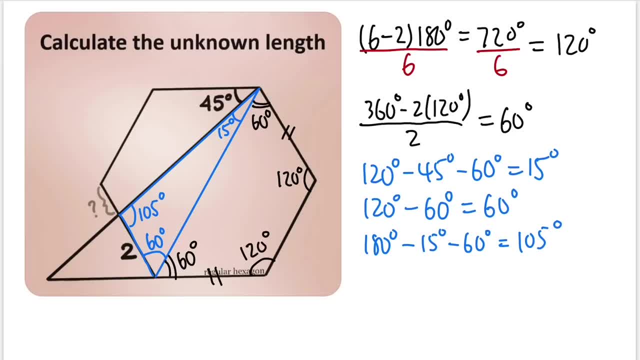 out the rest of the sides, and which side do we care, though? well, remember, we're trying to find out what this side is, and to help us out, i'm going to connect from here to here and i'm going to have a triangle, again in red, like this: 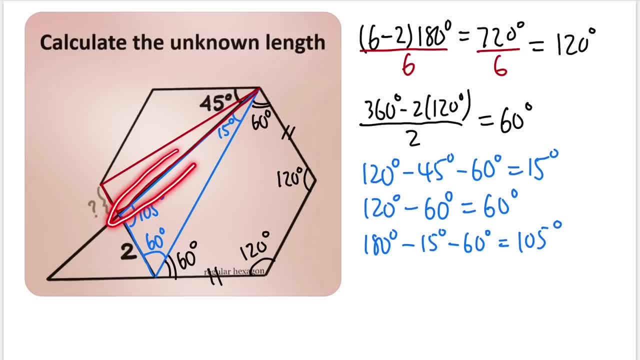 as you can see, we have one side that's in common for the blue and also the red triangle right there. so that side must be important, right? let me call that x and let's figure out what that is to do. so we will have to use law of sign, and i am just going to. 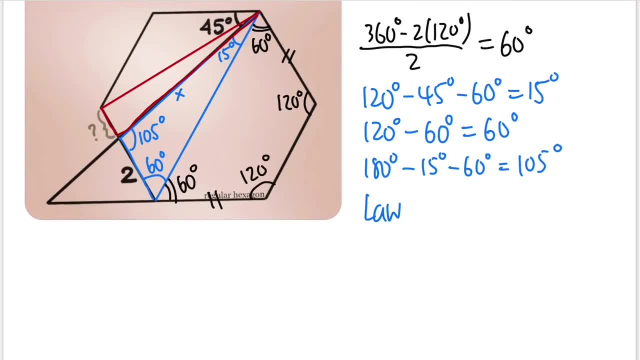 do a quick review with you guys. here is the law of sine which says: if we have a triangle, let's say we have angles a, b and c and then the corresponding sides, little a here, little b here and little c here. we know that sine of angle a over little a equals. 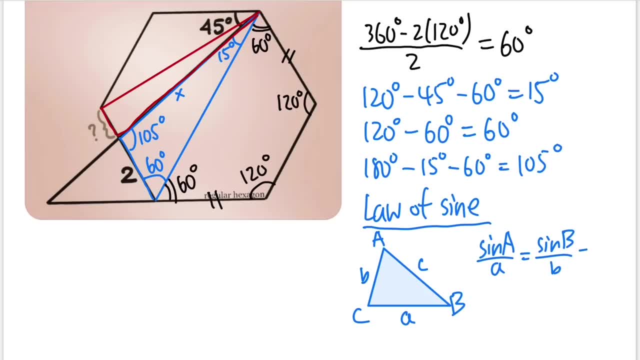 sine of angle b over little b. and then we can also do the same for sine of angle c over little c. here's a little secret for you guys: if you want to find out missing sides, do the reciprocals. it's easier. in another word: little a over sine of capital, a is equal to little. 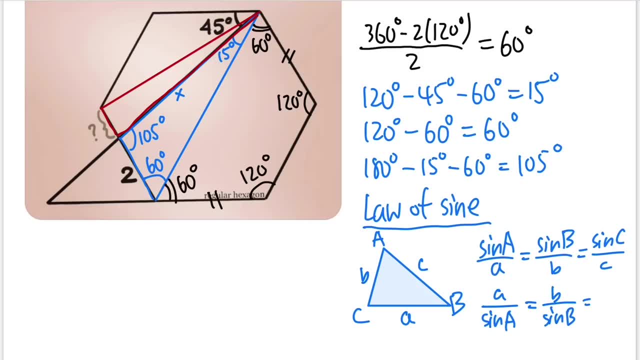 b over sine of capital b, and that's equal to little c over sine of angle c. it's easier this way. so now let's have a look. we have this side and this angle right, but we have to have to look at 15 degrees and also the two, because 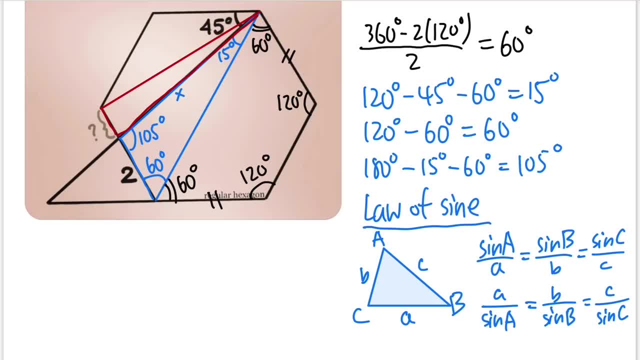 two is the only one that we know. so check this out. by law of sine, we know that x over sine of 60 degrees must equal to two over sine of 15 degrees, and i'm not going to simplify anything until the very end, right here. i'm just. 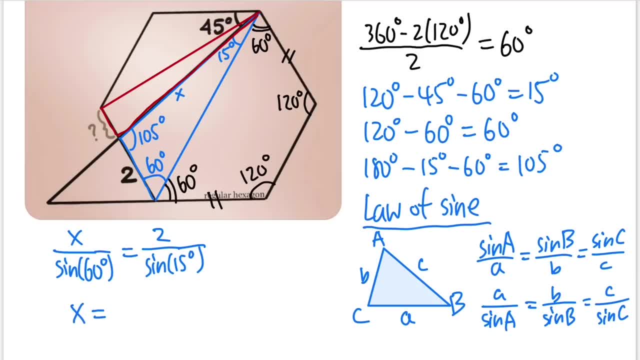 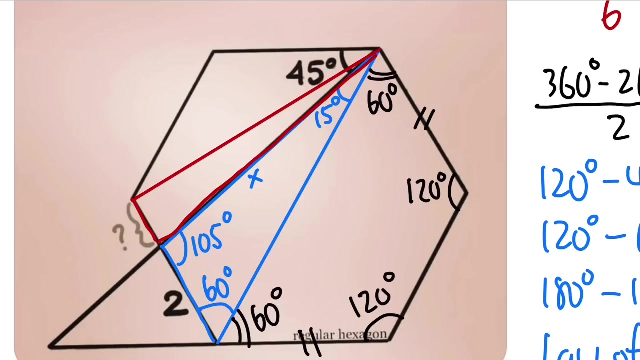 going to tell you: x is equal to multiply sine of 60 degrees on both sides. so we have 2 sine of 60 degrees over sine of 15 degrees. so that's what x is now. we know x already. let's go back to the picture, especially for the red triangle. let's figure out the missing angles. do we know about? 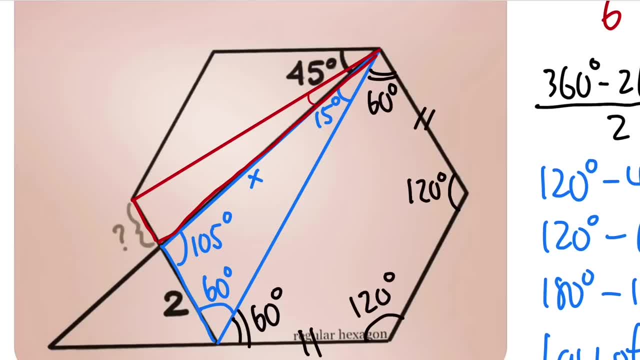 this angle here? yes, we do, but what is it? well, be careful. we will have to look at this top triangle here real quick. firstly, though, we know that this side it's the same as that side because, again, we have a regular hexagon, and this angle here is 120 degrees. so that means what for this angle? 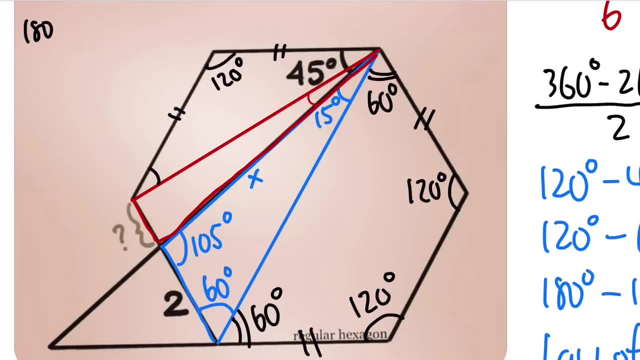 just go ahead and do 180 minus and we get 30 degrees, right. i saw this triangle. the base angles are the same, so this is 30. so that means this part here is 30 degrees, meaning that the red one here is 15 degrees. 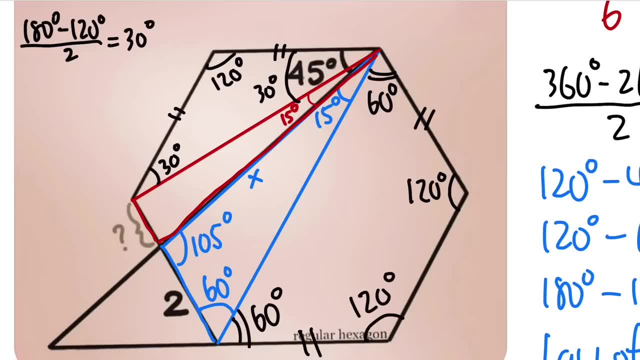 okay, and you know what? this is really cool because the whole thing from here to here should just be 120 degrees. be 120 degrees, right, and we know this right here is 30 degrees already, so let's just go ahead and do 120 degrees minus 30, which is 90 degrees. in fact, we have a right triangle here. now check this. 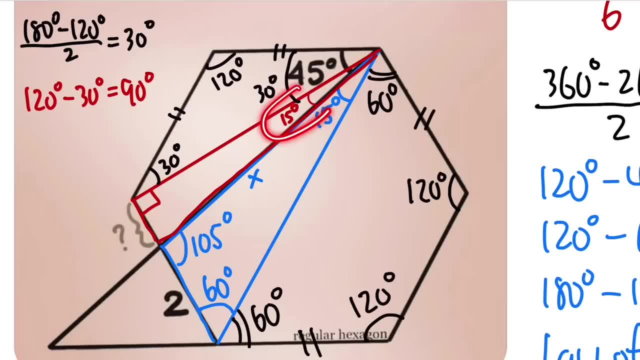 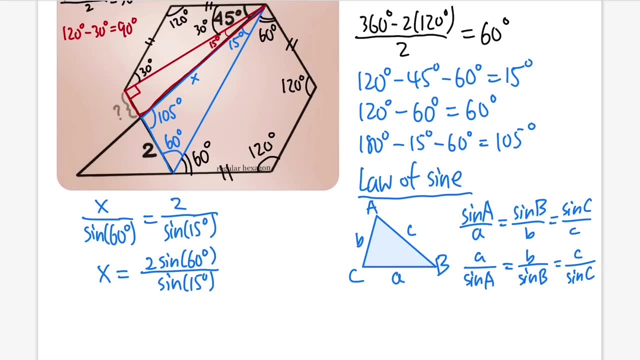 out. we actually have a right triangle. this is 15 degrees, and that's the question mark that we don't know, and we know the hypotenuse of the right triangle, which is x. so i am actually going to finish this right here for you guys. all we have to do is that we know sine of 15 degrees. 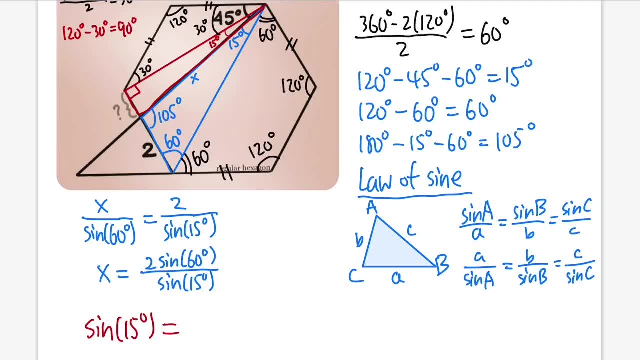 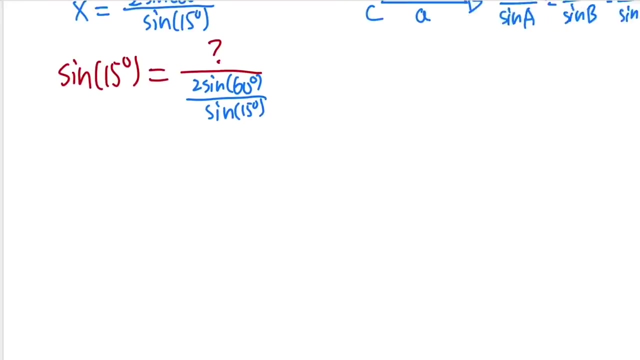 must be equal to opposite, which is the question mark over the hypotenuse which is x. so i will just write down question mark over the hypotenuse which is 2, sine of 60 degrees over sine of 15 degrees. now just focus on this. multiply the denominator on both sides, then we will see the question mark.